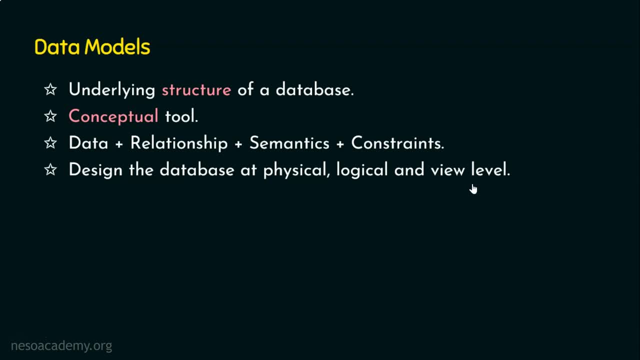 the physical level. two. the logical level. three. the final one is the view level. We are done with the basics of data model. Let's now see the various categories of data model. In this presentation, we are going to focus on four different categories of data model. The first: 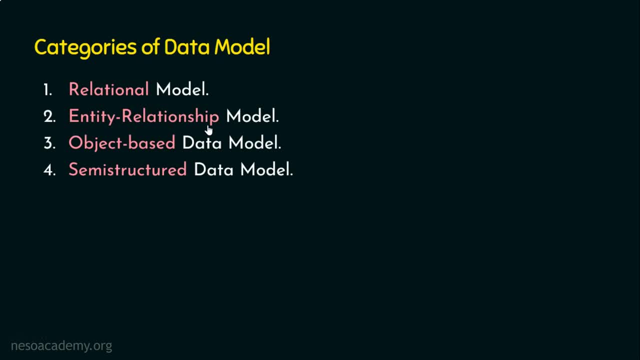 one is the relational model, The second one is the entity relationship model, The third one is the object-based data model and the last one is the semi-structured data model. Of course, we have other data models as well, but in this presentation we are going to focus only on these four data. 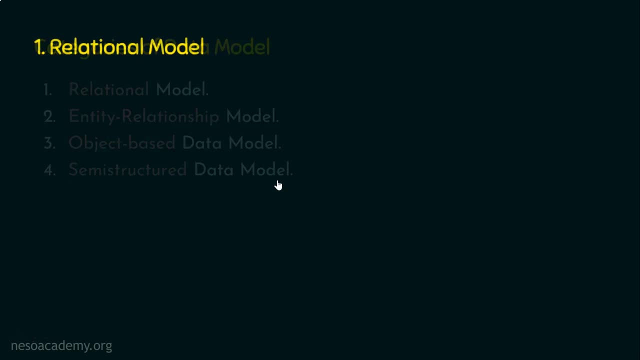 models. Let's start with the first data model, the relational model. Basically, a database is a collection of tables and we know this table is going to collect or store the data and these tables are also going to establish or maintain the relationship among the tables. So what does? 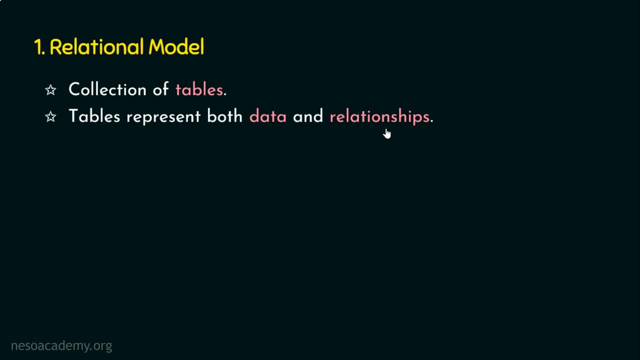 mean by this? See, we are going to store the data in databases, where databases are collection of tables, and these tables are going to store the data in the form of rows and columns. Let's say we have two tables: One is the student table, other one is the instructor table and this student table. 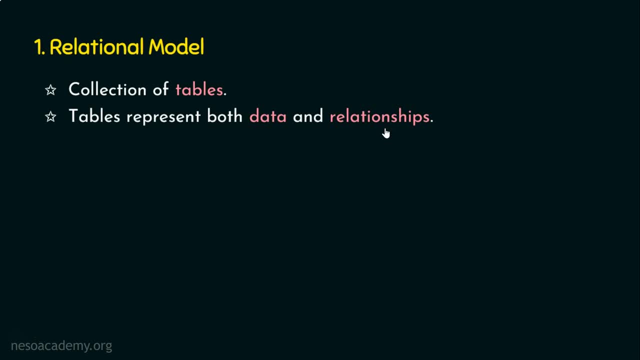 is going to contain the information about the student and obviously the instructor table is going to store the data about the instructors. Now, obviously, student and instructor are somehow related, isn't it? The relationship is also a table In this case. so in relational model, everything is of tables. The data are obviously going to be. 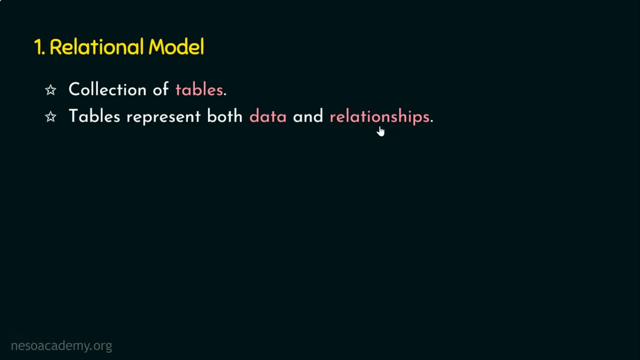 stored in the table and the relationship are also represented in the form of tables. No worries, when we see some examples, you will be able to understand things. So in relational model, everything is represented in the form of tables and we know basically a table is going to contain. 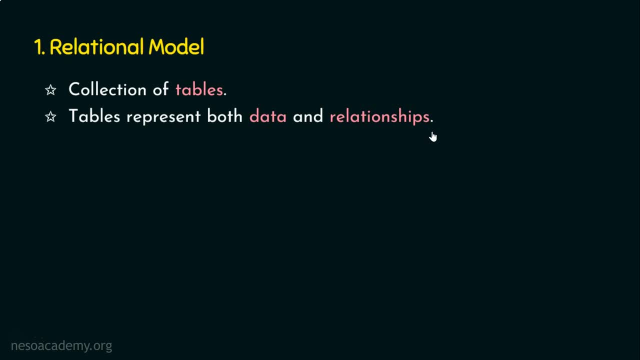 multiple columns and each column in the table will have unique names. Likewise, in a database, we may have multiple tables and each table will have unique names. So in a database, we may have a database and each column will have unique names. So in relational model we have multiple columns. 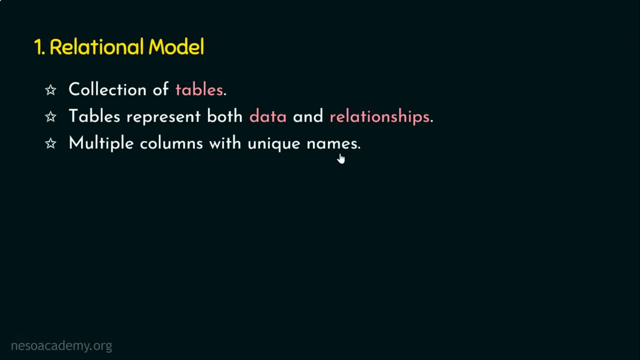 in the table with a unique names, and we may also have multiple tables with a unique name in a database. Now why it is named as a relational model? Because in RTBMS, the relational database management system, we refer tables as relations. because in relational model. 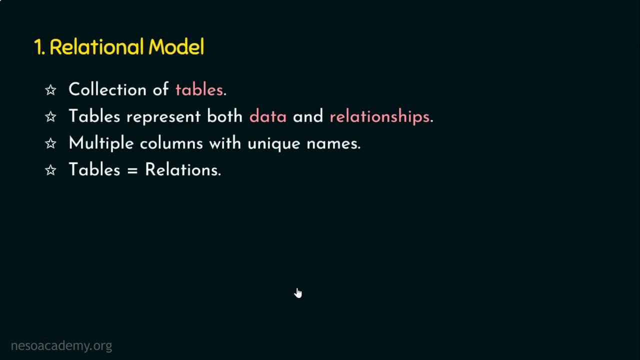 everything is of relation. Obviously, the data are going to be stored in the relation or table only, and the relationship among the data or the relationship, the table, is also going to be stored in a relation only. and this relational model is also referred as a record based model. and what is a record? it is actually a fixed format: records of several. 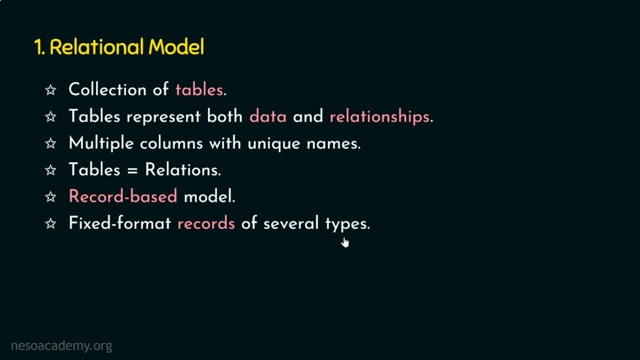 types of several data types. i will explain about this when we see an example. so in simple terms, relational model is also referred as a record based model. and what is a record actually? each record defines a fixed number of fields or attributes. say, if we say something, as a record? 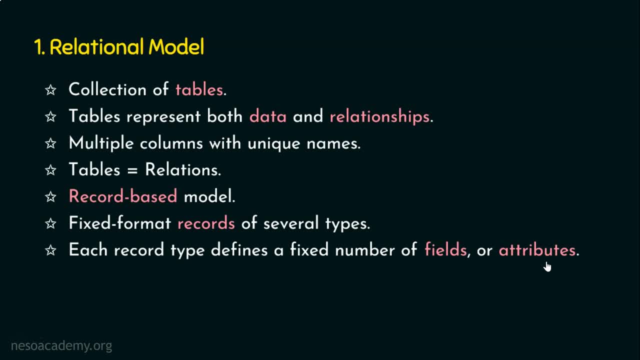 each record is going to have a fixed number of fields or attributes. don't worry about this now. in the next slide we are going to see some examples now. is this model widely used? yes, this relational model is the most widely used data model in this contemporary world. 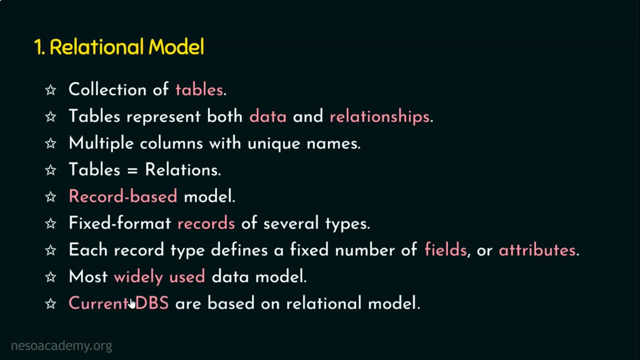 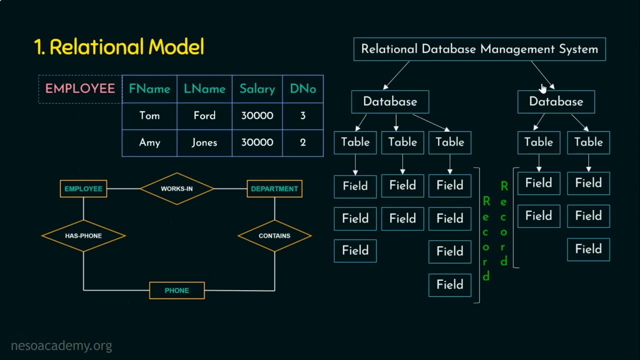 so when i say this is the most widely used data model, obviously the current database systems are based on the relational model only. So we are done with the basics of relational model. Before we step into the next data model, let's see an example. Let's say this is the relational database management. 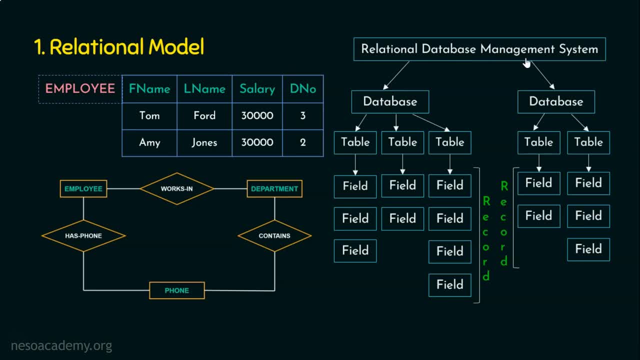 system, or simply RDBMS, where this database management system is a collection of databases and we know databases are actually collection of tables and we know a table is a collection of various fields and the collection of various fields are referred as the record Say. if we 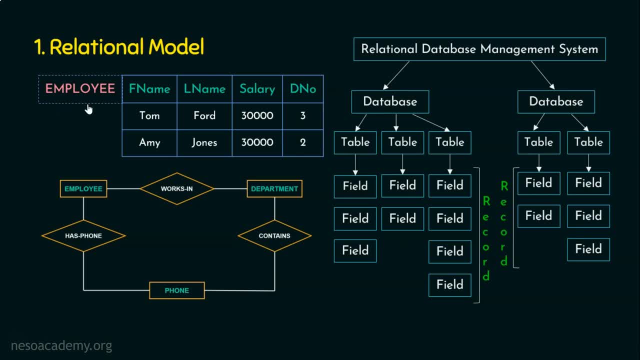 talk about an employee relation or an employee table. let's say, this employee table contains four attributes or four columns: first name, last name, salary and department number. And this particular relation has four columns or four attributes: the first name, last name, salary. 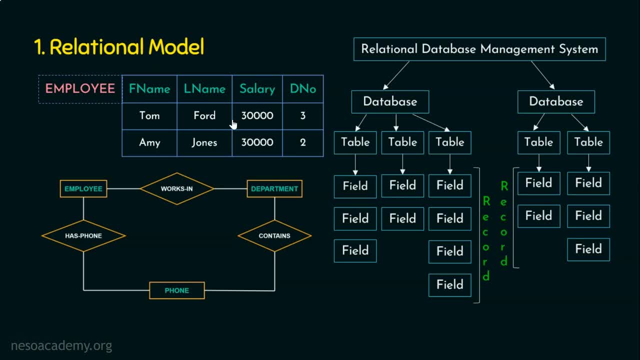 and department number. Can you see here, Tom Ford, 30,000 and 30,000.. And this particular relation has four columns or four attributes: the first name, last name, salary and department number. Can you see here, Tom Ford, 30,000 and 30,000.. This complete. 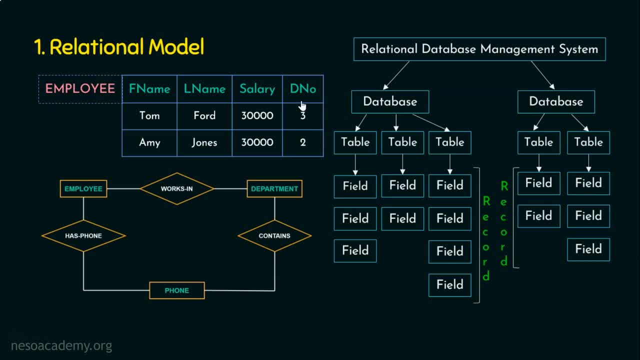 information are referred as a record, where this record is actually having four fields: the first name field, the last name field, salary and department number fields. So, in simple terms, a record is a collection of fields and collection of fields are referred as a table and collection. 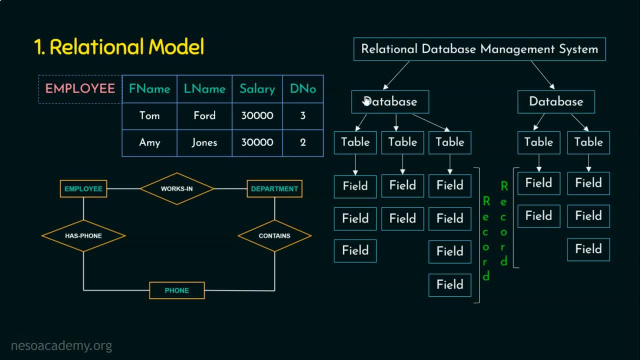 of tables are referred as database and collection of databases are referred as the relational database management system. So, in simple terms, in relational database system, multiple relations are there. Each relation is actually a table and each table will contain multiple fields and the collection of 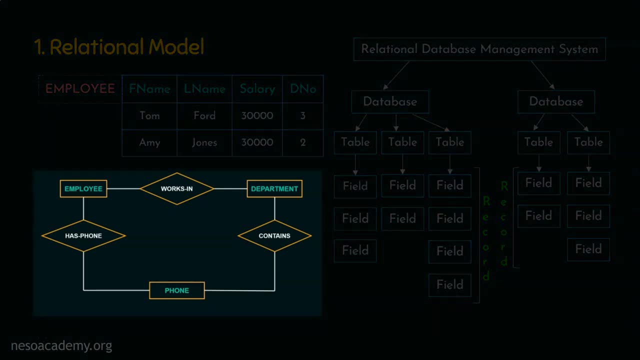 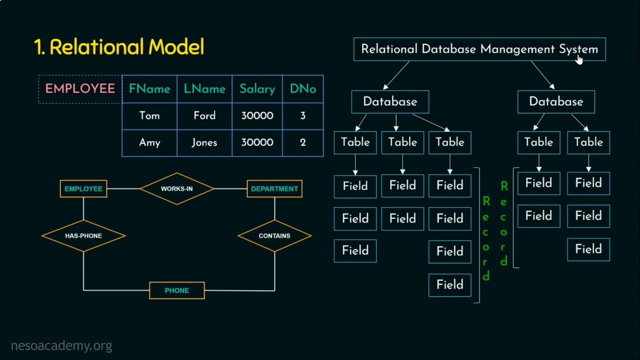 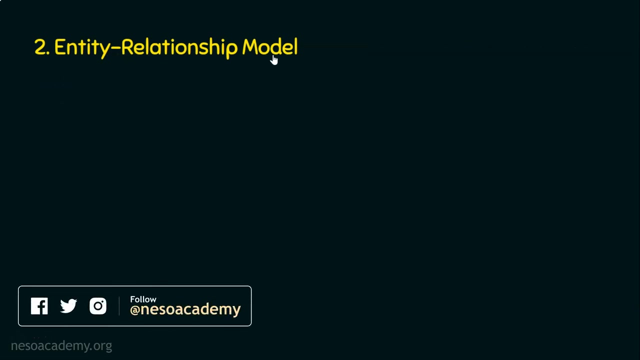 fields are referred as records. We also see a diagram here. Don't worry about this now. In the next data model we will see about this. So we are done with the first data model, the relational data model. Let's now move on to the next data model, the ER model, the entity relationship. 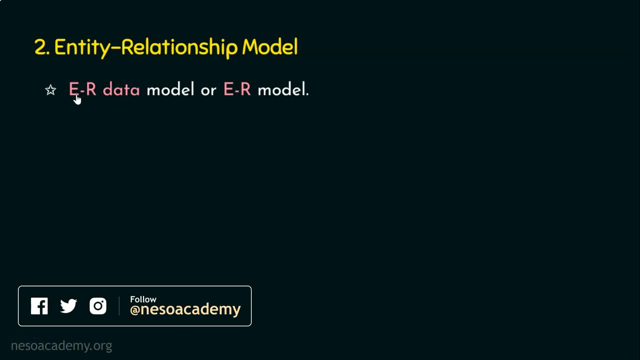 model. So this entity relationship model is also referred as the ER data model or simply ER model. So E stands for entity, R stands for relationship. What do we mean by this entity We know? basically, this ER model is actually a collection of basic objects, and these objects 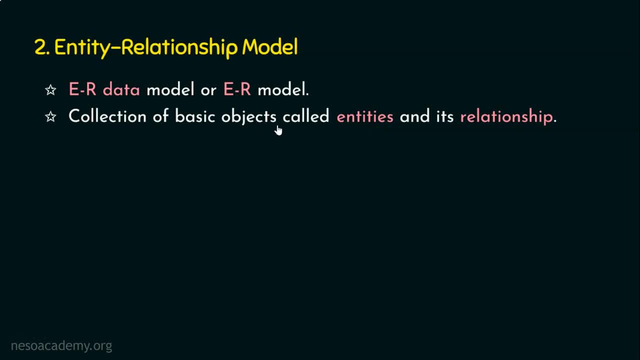 are referred as entities and when we say this is a collection of multiple entities and obviously there will be relationship among entities, right? So there will be a relationship among student entity as well as instructor entity. and when we say this entity is a collection of basic objects, 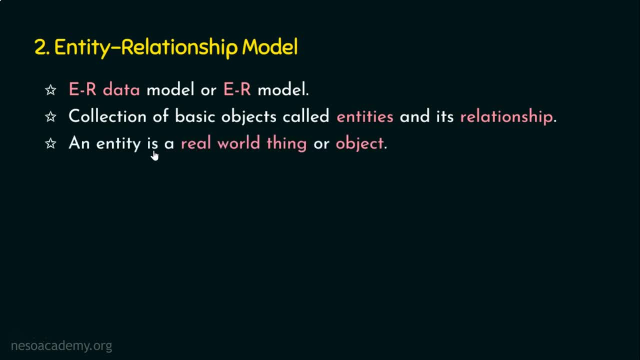 these objects are real world entities or real world things. right, So we can say: an entity is a real world thing or object, And when we say that this entity is a real world thing or object, obviously each entity or each object is distinguishable from other objects. 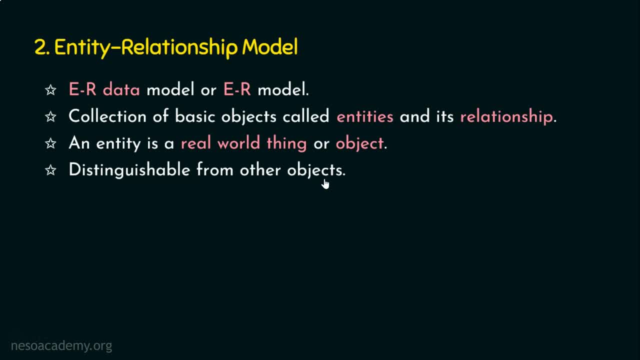 Now is this ER model is widely used. Yes, like relational model, ER model is also widely used. But the important thing to note here about the ER model is this ER model is widely used in the database design. before you start creating the database, before you start creating the table, 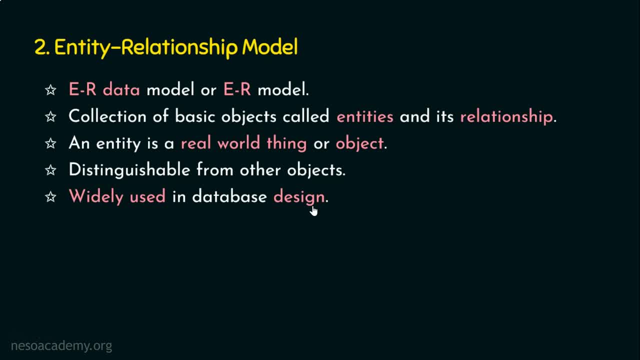 we are going to use the ER model in order to design the database. In the previous data model, I mean the relational model. the current database systems are actually using the relational model, Whereas here, the second data model, which is the ER model. we are going to use this ER model for. 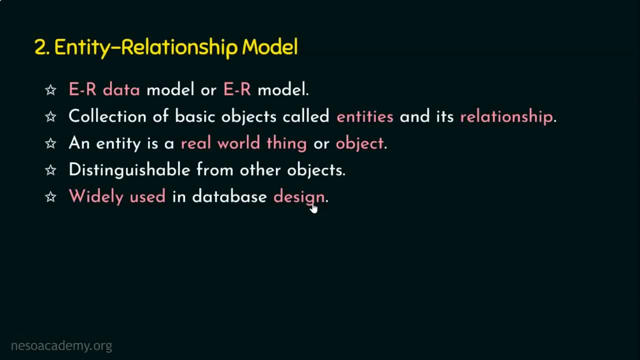 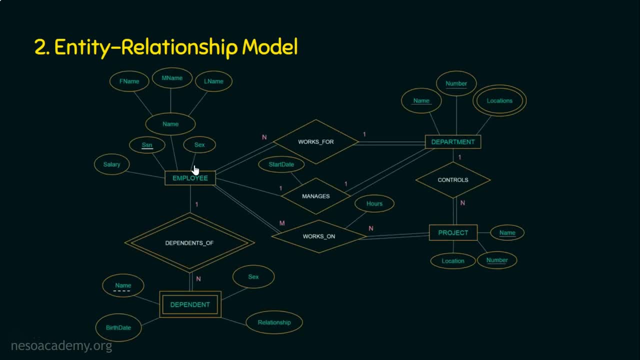 designing the database. Let's see an example, then it will be easy for you to understand. Here is the example of an ER model. Can you see here everything is referred as an entity. This employee is an entity, dependent is an entity, project department are entities, and each. 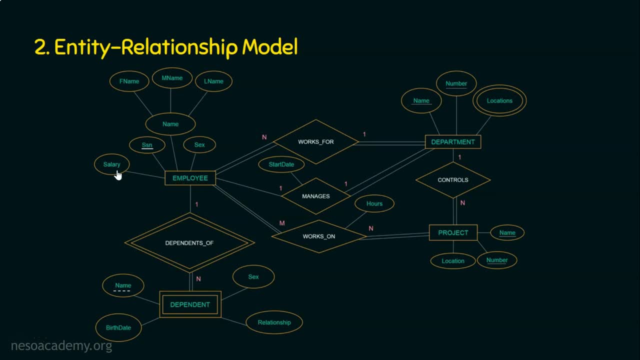 entity or each object is described by some attributes: salary, SSN name, gender or sex. and name attribute has three more sub-attributes: the first name, middle name and the last name. So don't worry about this ER model. now, Anyway, in the next chapter we are going to 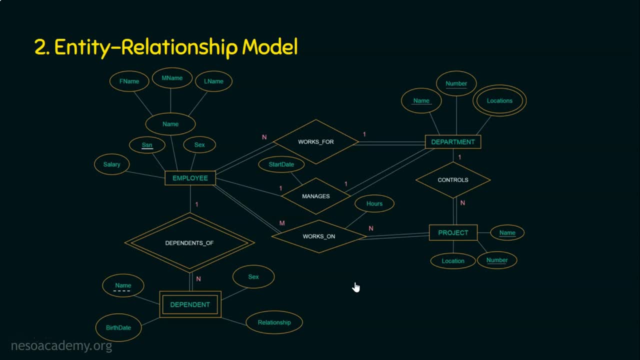 exclude the ER model from the database. So let's see how we are going to do this. Let's exclusively focus on the database design aspects, where we are going to see about the ER model. We are going to see various examples about ER model. So for now, just understand this ER. 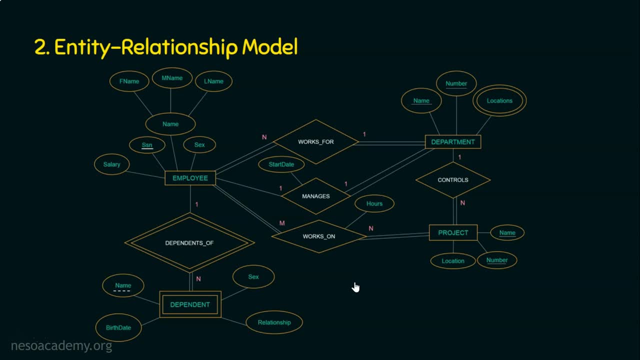 model is a schematic or diagrammatic representation so that this can be used for designing the database. And also, please be noted here that this entity is related to other entity through some relationships. Can you see here? this employee entity has some relationship with other entities like department and. 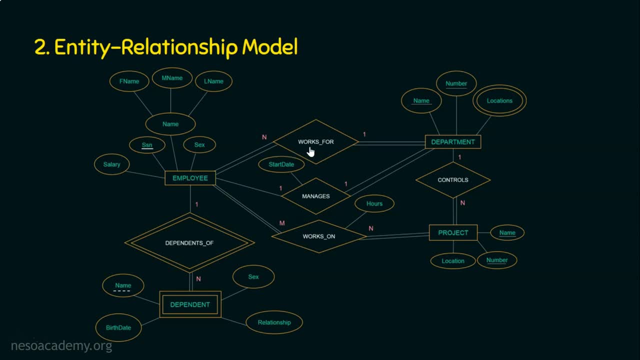 project And what is the name of the relationship This employee works for, department this works for is a relationship. this manages is a relationship. works on is also a relationship. So this is an entity. these are all attributes and these are all the relationship. No worries. 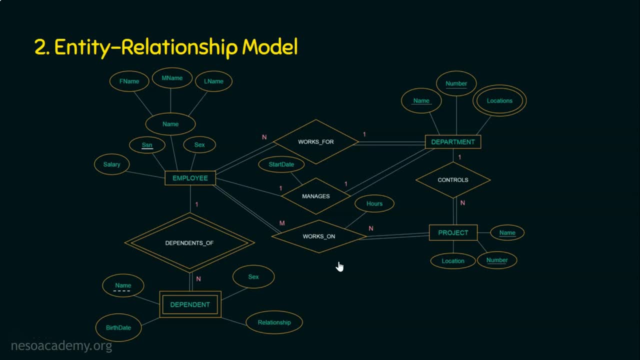 about the terminologies used. we are going to exclusively focus on the database design aspects in the next chapter. So we are done with the second data model, the entity relationship model. Let's now move on to the third data model, the object-based model. We know object-. 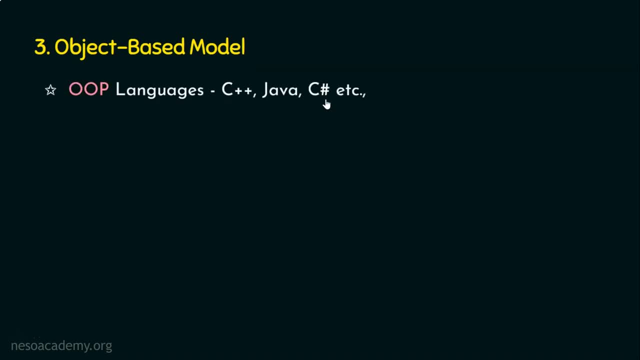 oriented languages like the C++, Java, C, Ash or C Sharp. We know these are all the object orientated programming languages. Suppose, if our front end is designed using object- oriented programming language, we need to have the back end which also supports the 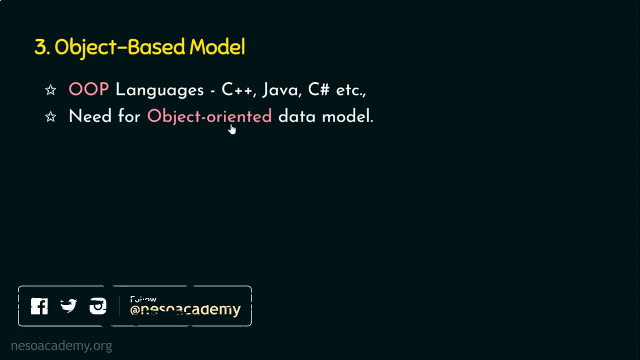 front end right. So in that case we are in a need for object-oriented data model, and that is why we are ending up here with the object-based model where this object-based model is actually used, the ER model, with the object-oriented features In the previous data model. we have seen about the 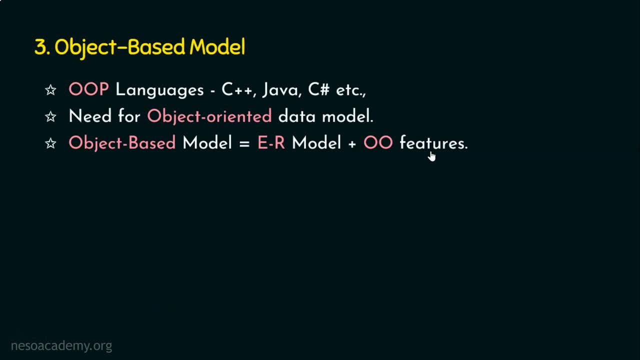 entity relationship model, where we have seen everything is of entities, where each entities are referred as an object, which are real world entities or real world things, and each real world entity, the objects, are distinguishable from other objects. So what we are going to do here is in the 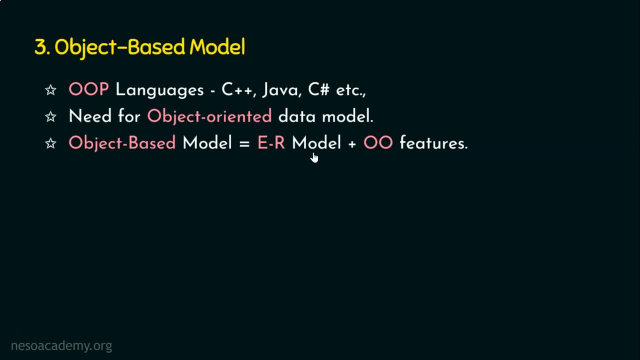 object-based model. we are going to make use of the features of the ER model, along with the object oriented features like data encapsulation, inheritance, etc. We also have a variation of the object-based data model, which is object-relational data model. where this object-relational data model 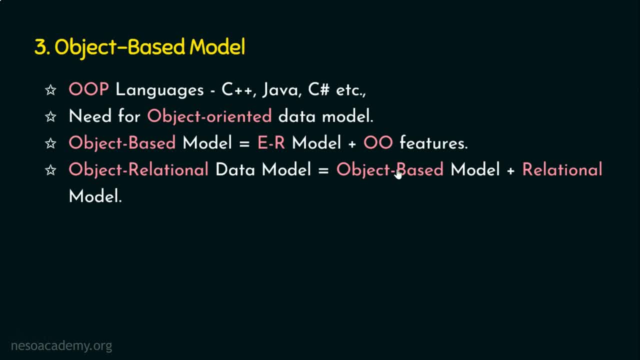 which is the combination of object-based model, which is this along with the relational model, which is the first data model we have seen Object-based model. when it is combined with the relational model, we get object-relational data model Before we step into the fourth data model. 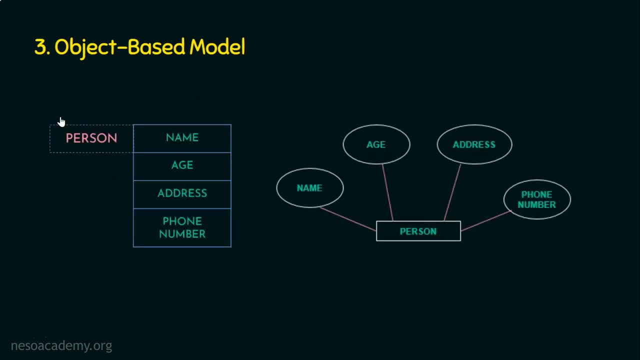 let's see how it works. Let's see the example. So in this example we can see that this is an object. Person is an object which contains attributes like name, age, address and phone number. So this can also be represented as an ER representation. This is an entity or an object person which contains attributes like 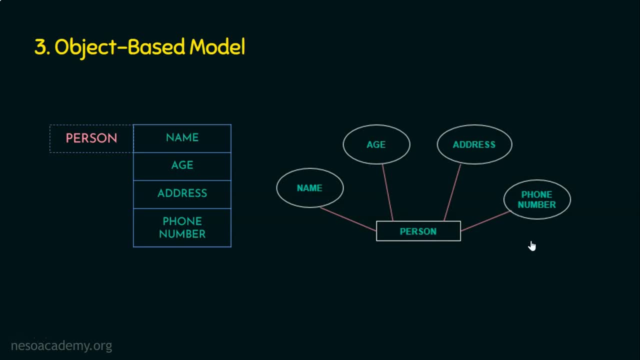 name, age, address and phone number. So don't worry about this now. when the course progresses, we will be able to understand things clearly. So we are done with the third data model, the object based model. Let's see the last data model, the semi-structured data model. The name itself says: 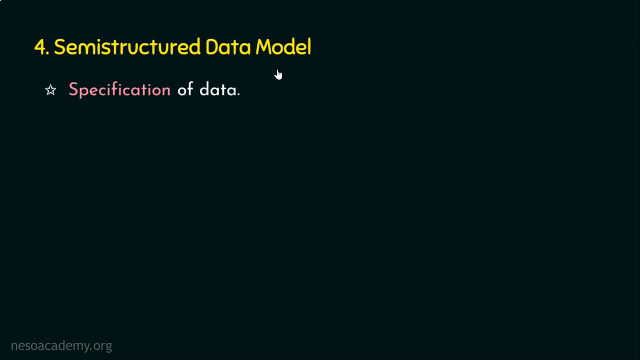 that this data model is already semi-structured. It means it's going to deal with the specification of the data. What do we mean by this? It means the individual data items of the same type may have different sets of attributes. What do we mean by this? This data model is mainly used. 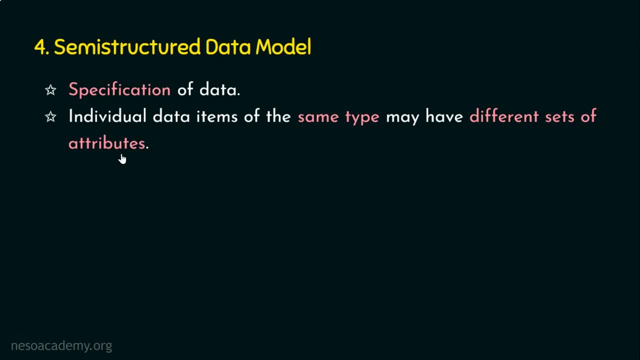 for transferring the data among applications, Say, if there are two different applications and data transfer needs to be done, Obviously data needs to be stored somewhere right In the database. if we use semi-structured data model, then transferring the data among applications is also easier. No worries, in the last phase of this subject we are going to exclusively 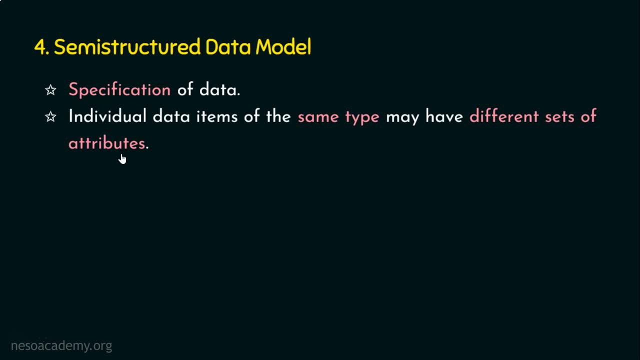 focus on a special language, the extensible markup language, where we will be understanding clearly about this semi-structured data model. So for now, just understand two different applications need to communicate with each other. So let's see the last phase of this subject And if they want to use the databases, then we can go for semi-structured data model where it. 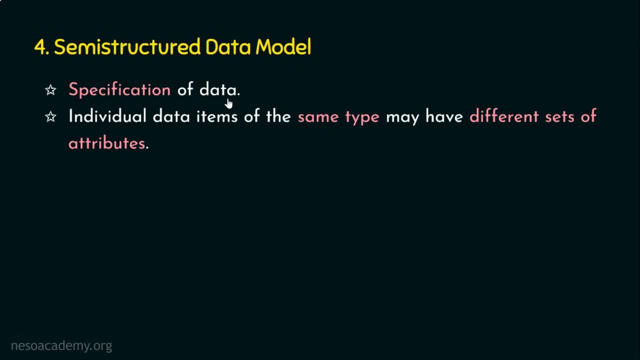 deals with the specification of data, And we can clearly witness that this is contrast to the previous data models we have seen. I mean, this is contrast to the previous models, like the relational model, the entity relationship model, or simply ER model, and the object based model and the language. 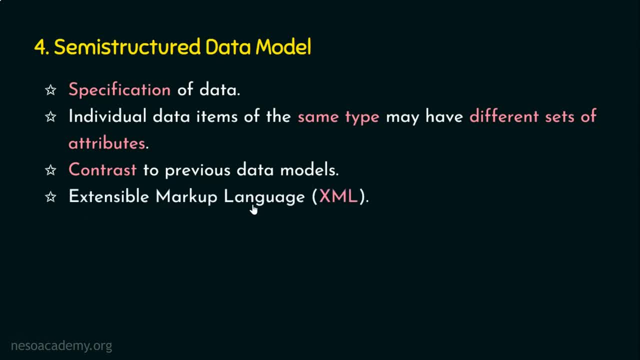 that supports this semi-structured data model is the extensible markup language, simply XML. Before we see the language that supports the semi-structured data model, is the extensible markup language, simply XML. the other data models: Let's see an example for XML, Say. here I'm going to create a note where 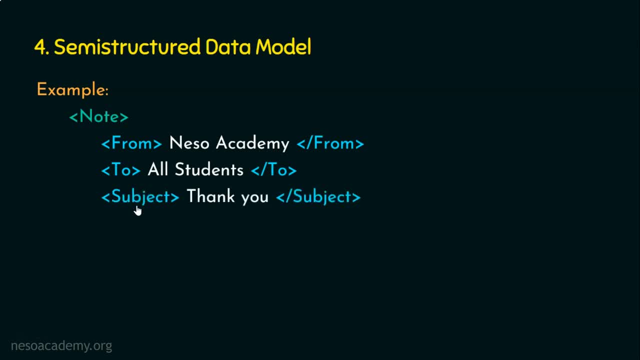 this note is from Neso Academy to all students, and the subject of this note is thank you, and the body of this note is: thank you for subscribing Neso Academy, good luck. And this body ends here. and this is the end of the note. Can you see here? this is like the HTML language, but the difference here. 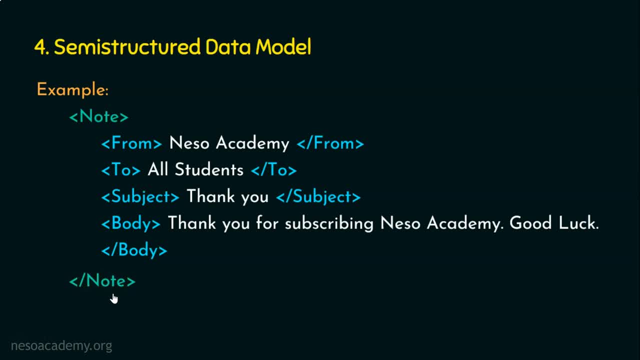 in HTML we have predefined tags. Here we can create our own tags. Can you see here? this is a note where I am creating my own tag. this is a note. This note has a from field or a from tag, So this from: 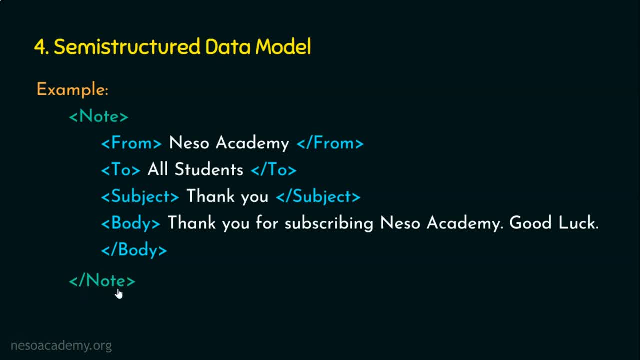 is a user-defined tag. This to subject body and note: all are user-defined tag. Can you see here the hierarchy or even the structure here? This note is the parent element and this contains sub-elements like from to subject body. 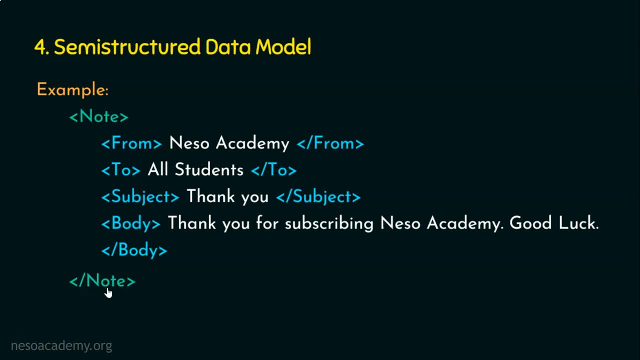 And this is the end of this note tag. I know things will be unclear at the moment, but for now, just understand the structure. This contains the data, which is Neso Academy. all students, thank you. thank you for subscribing Neso Academy, good luck. All these are the data that we are going to store. 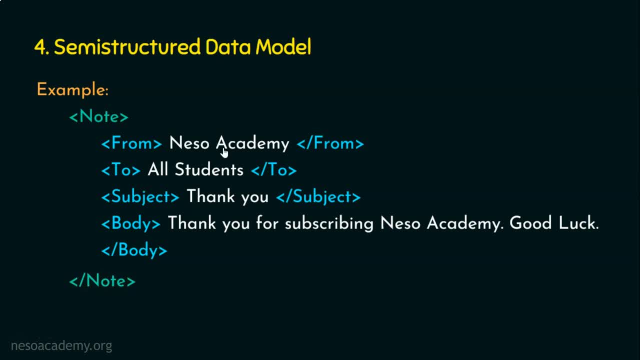 or transfer. At the same time, these data are also structured and this is how it is structured. The note is the outer element, or the parent tag, which contains sub-tags like from to subject body, And each data has its own structure. This data belongs to this from and this data is belonging. 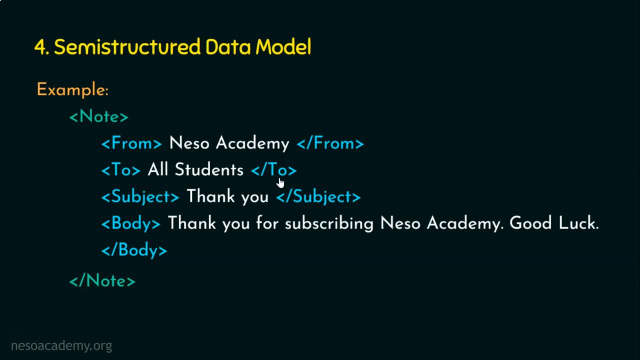 to to, And this is how data is actually structured and stored, And that's why we call XML is a semi-structured language, And this is what the point two of the semi-structured data model, which we have seen in the previous slide, says: We can have multiple nodes with multiple different.